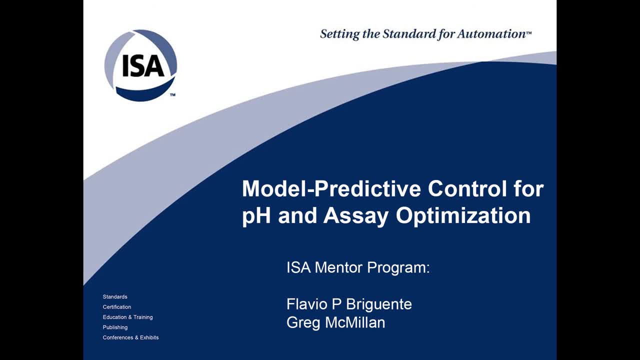 I'm glad you all could join us today. We are very fortunate to have Flavio Briguente do a presentation on his achievements in the use of a small model predictive control, And he has made some significant improvements in process operations as a result of using 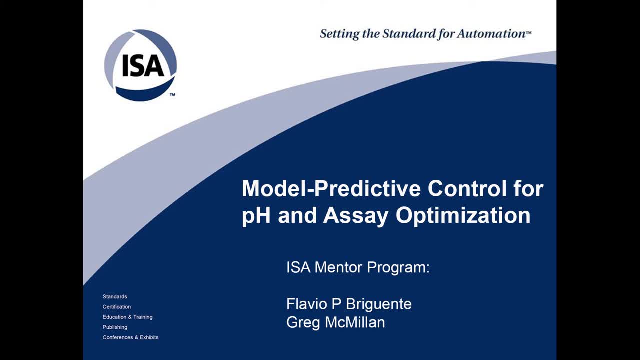 what is built into a DCS for doing small model predictive control. Flavio Briguente has been with the program for many years and is more like a resource than a protege, So we are really fortunate to have Flavio give us this presentation. So go ahead, Flavio. 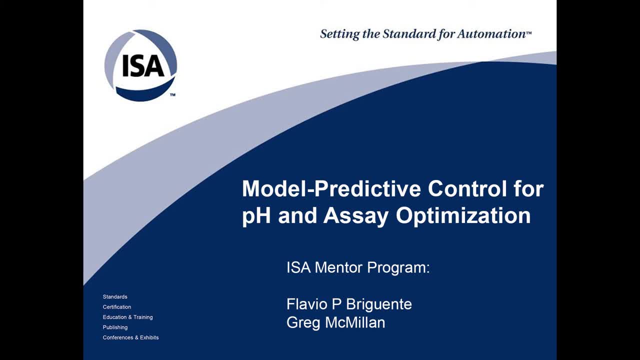 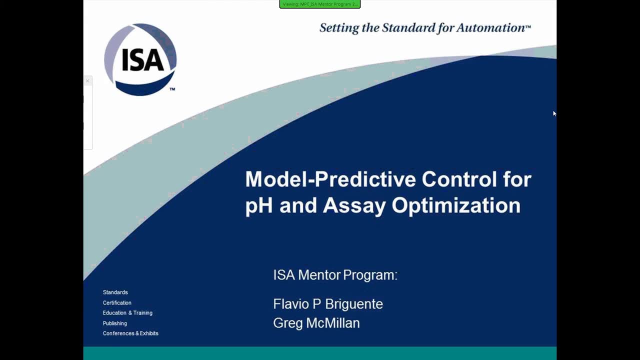 and share your file. Flavio Briguente MD. Okay, Thank you, Dr David Lambert MD. Thank you. So the idea here today is to give you an overview of a case study that was implemented in Brazil in the Monsanto site plan, in San Jose dos Campos, We implemented model predictive control. 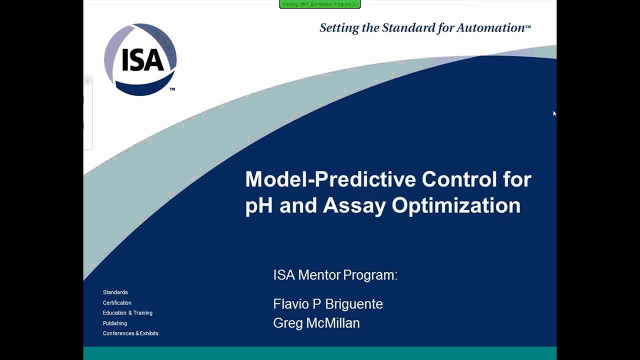 for pH and assay optimization. I also have support from Greg. During the mentor program in ISA. we… David Lambert MD. Thank you, Dr David Lambert MD. Thank you, Dr David Lambert MD. We always discuss a lot on the implementations on these cases. 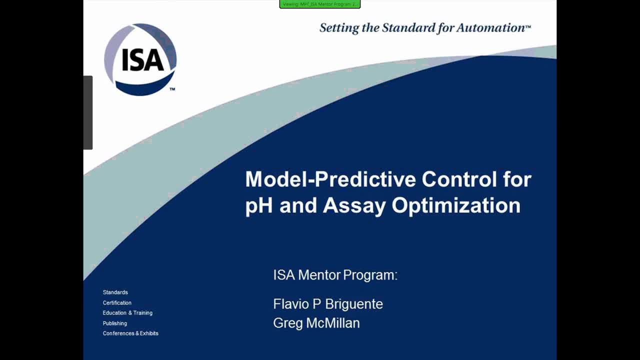 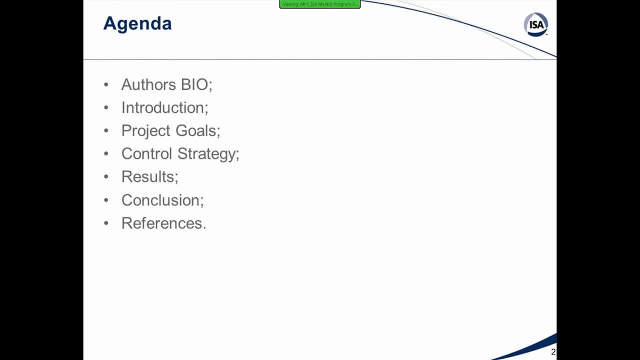 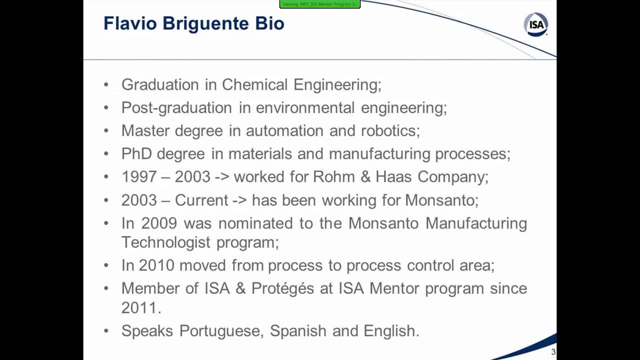 for industry, So I'd like also to thank Greg for supporting me on this project. The agenda today is going to cover these topics. So, talking about myself, I'm a chemical engineer with about 20 years in the chemical industry. Dr David Lambert MD. Okay, Thank you. 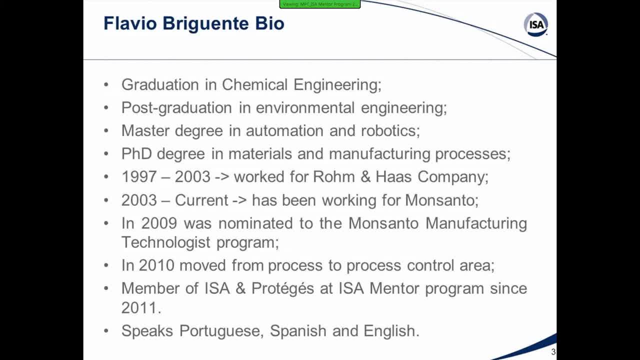 Dr David Lambert MD. Thank you, Dr David Lambert MD, Thank you. I started in 1997 working for Haman Haas Company. In 2003, I decided to move to Monsanto And during this period I got my post-graduation in environmental engineering. 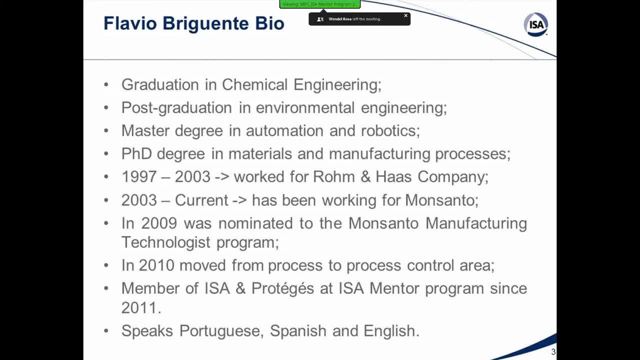 Got also a master degree in automation and robotics And recently a PhD degree in materials and manufacturing processes. In 2009, I was nominated in TS to the Monsanto Manufacturing Technologies Program. It's a technical career within Monsanto. In 2010, I moved from process engineering to process control area. 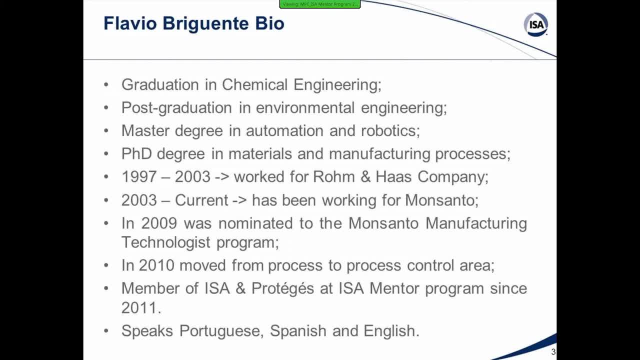 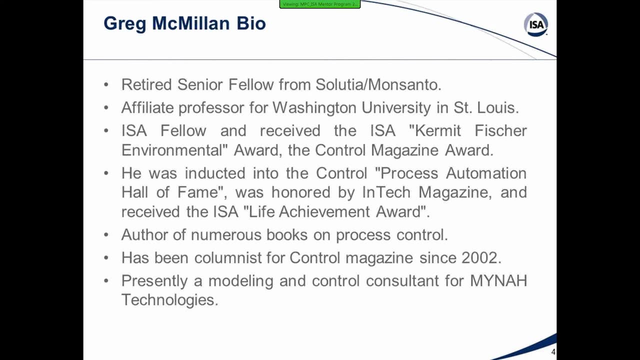 And I'm a member of ISA and protege at ISA mentor program since 2011.. And, And I speak Portuguese and try to speak English and Spanish. so Greg is a retired senior fellow from Salesian and Monsanto. Worked for about 35 years for both companies. 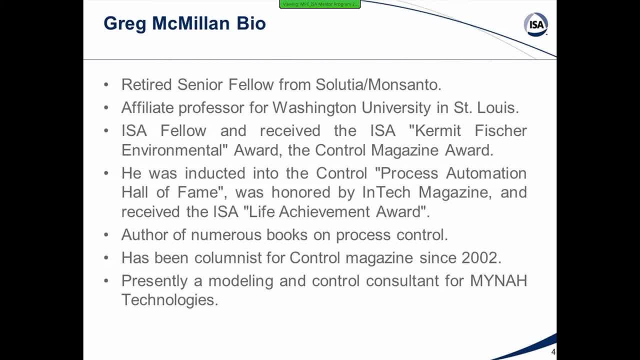 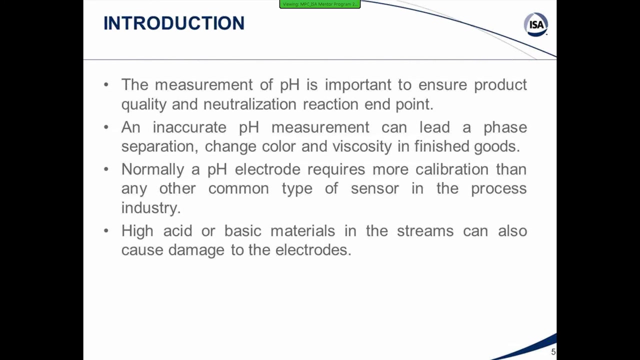 And he's an affiliate professor at Washington University, ISA fellow and received many awards, Is out there of numerous books on process control And has- He's presently now a modeling and control consultant for MENA technologies. So, Talking a little bit about 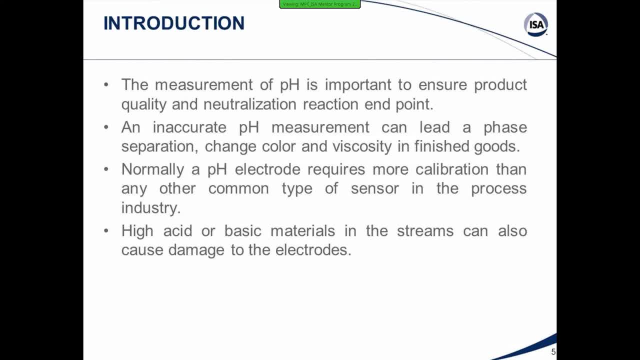 This is an important measurement for the industry in general, Mainly because to ensure product quality and also, in some cases, to detect and eliminate. to detect the endpoint of a neutralization reactor, neutralization reaction. So an accurate measurement of pH really can let the products to be within certain range. 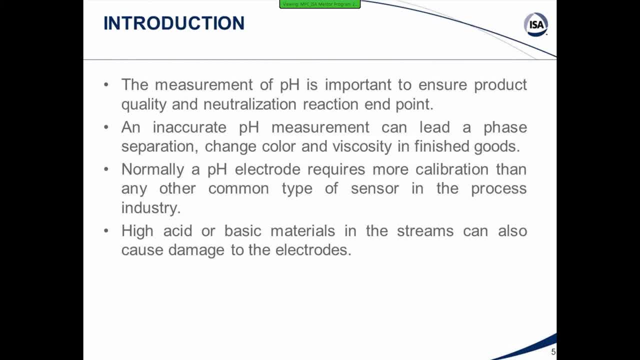 of specification and avoid kind of problems like phase separation, change in color and viscosity when they are placed in the market. So normally pH electrodes require more calibration than other common type of sensors in the industry And also for processes that handle high-acid or basic materials on the streams it can. 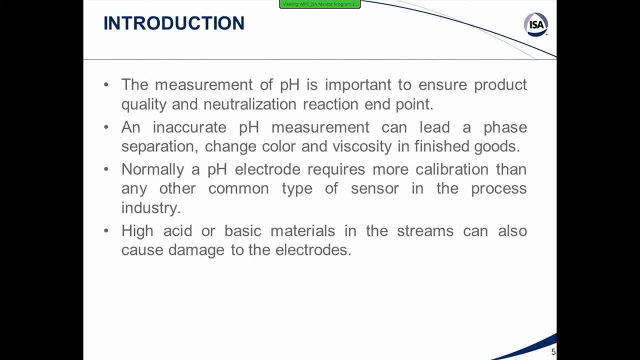 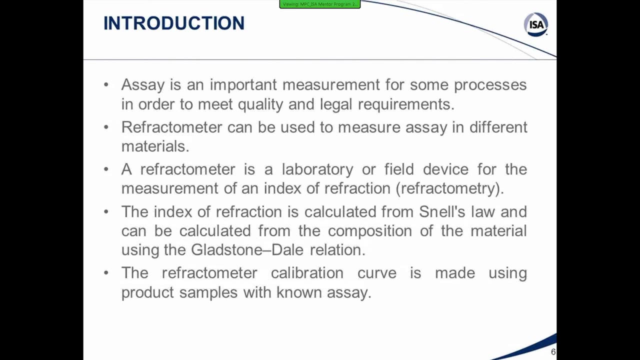 cause damage to the electrodes, So the maintenance is essential for good operation. when we talk about pH measurement Technology, A little bit about assay. it's also an important measurement for some process, because not only for meat quality requirements but also legal requirements, especially when you talk about 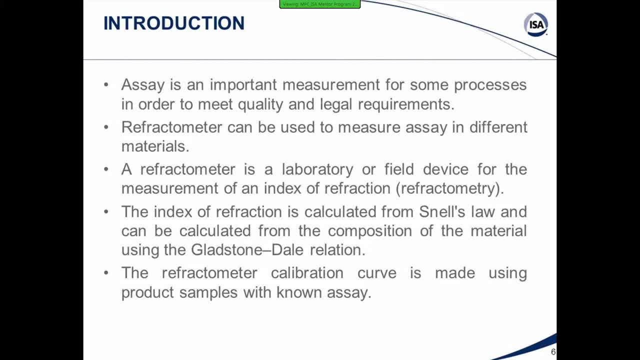 active ingredients for some formulations. So a refractometer can be used. it's a device that can be used to measure assay in different materials. So you can use either both lab. There are a few devices for measuring the index of refraction that we call refractometry. 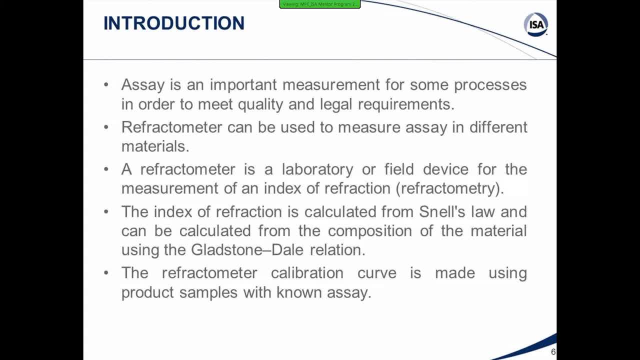 So the index of refraction is calculated from the law and can be also calculated from the composition of the material using the Glaston-Dale relation And, in a practical way, the calibration of a refractometer. we just made a curve. 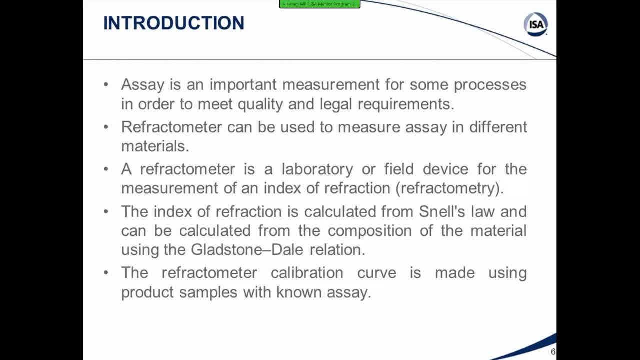 It's a curve And it's a range, So we can use it for a certain range of mass, And we can also use it for a specific range of mass. So we can use it for a specific range of mass, We can use it for a certain range of mass. 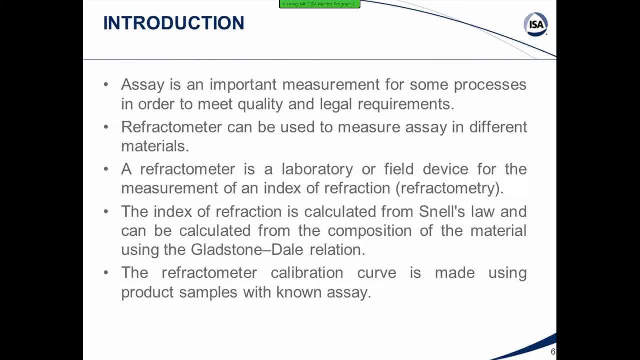 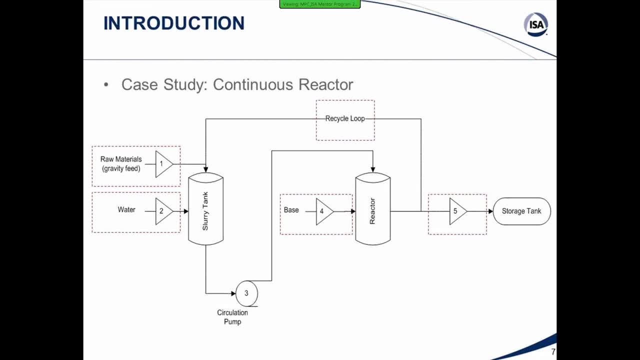 And we can use it for a specific range of mass, Using the product samples with very no assay, And then you can get – and for a certain range in your process to make also the measurements accurate. So in the case study we are talking about a continuous neutralization reactor. 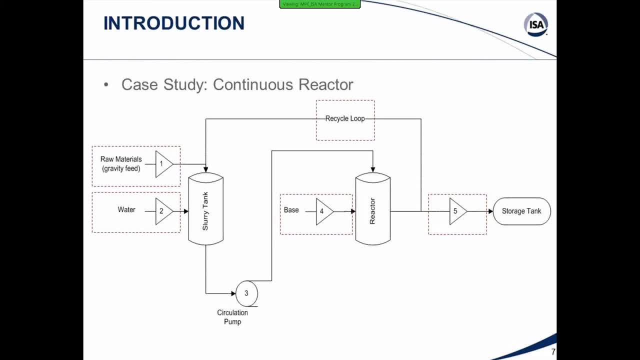 So first of all, we have two tanks in the system. The first tank is called the slurry tank. It's the tank where we charge water and keep feeding water continuously And also we feed a solid material that's being added by gravity. 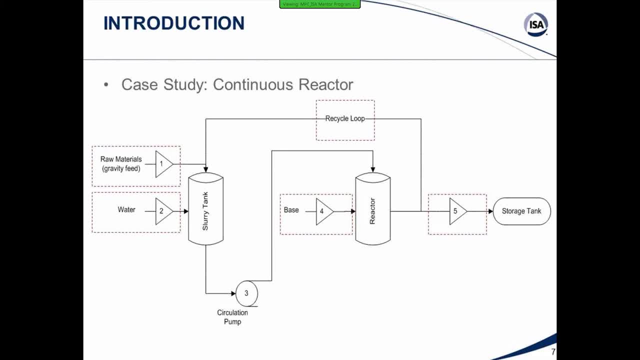 In this case we have an enough valve that open and close at a certain frequency just to feed product into the slurry tank. This tank is controlled, The level of this tank is controlled, So we keep around 60 percent. Then the slurry is pumped to the reactor – it's the second tank on the screen – and where 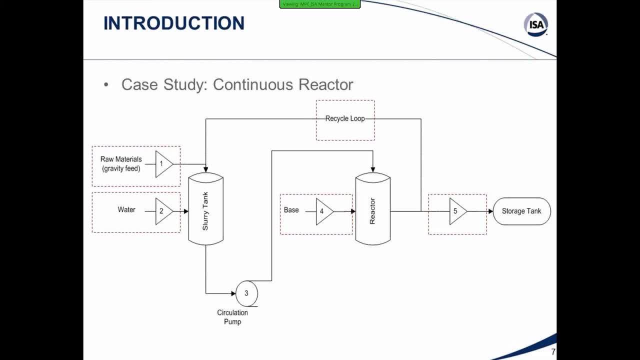 we add a base to neutralize the acids and also make the final product and send it to the storage tank. So part of this product is recycled, It's in the recycle loop and goes back to the slurry tank to ensure a minimum concentration of product here to keep actually a continuous flow rate or continuous production. 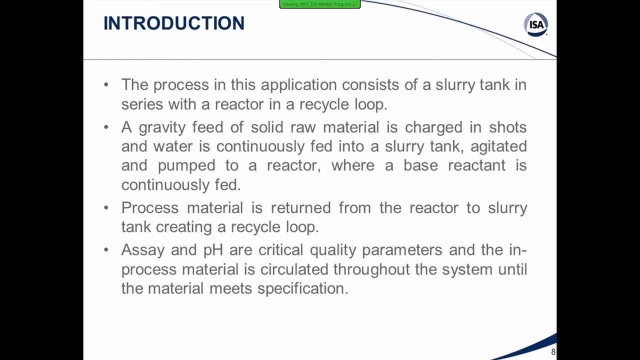 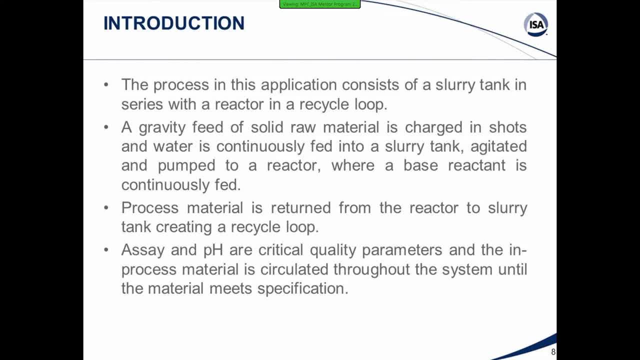 We're going to go back to the slurry tank, We're going to go back to the slurry tank And we're going to go back to the slurry tank, So it's always going to be in the slurry- And also to allow the product to be transferred downstream from the storage tanks we need. 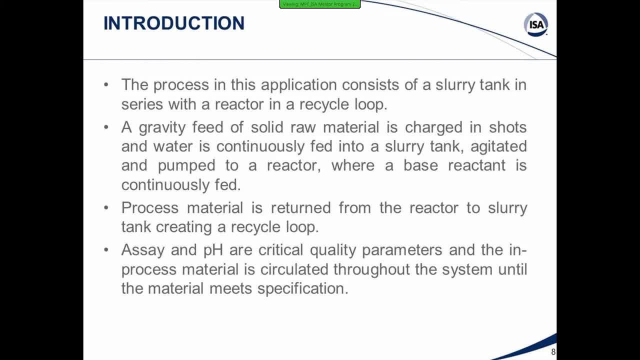 to control it within a certain range, according to the product specification, And because of that we define our – we set our production rates to get them as stable as possible. the process and the flow rates to avoid upsets and downtimes in the system. so 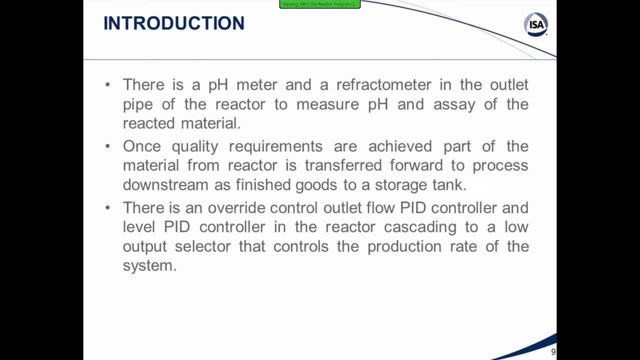 the page meter and refractometer is placed in the outlet pipe of the reactor and and this information is used to for sending, transferring the automatically the product downstream. so in the past there was a kind of PID control that they used to to do this kind of pH and S a control. we tried many 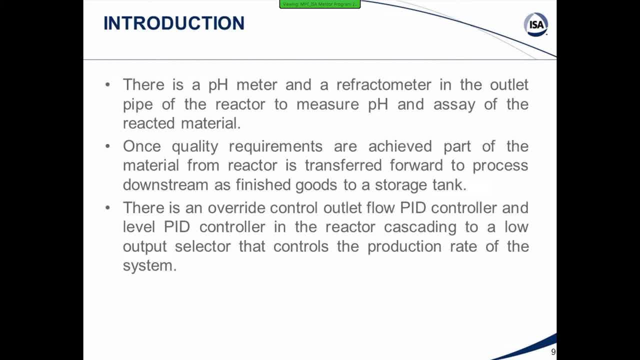 many actions to reduce variability using PIDs, but as it, this system works from multi-purpose way. we run more than one product in the system and we can reduce variability. that is the most important thing to do system. the PIDs were not running properly, So then we decided to think about a new country strategy to improve those controls. 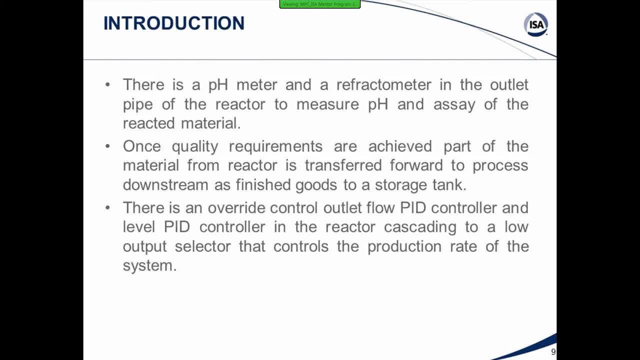 Also, in the tank there's an overhead control for level. So the operators are going to set the production rate. They're going to enter with the value they need to operate, But also in case the level of the system gets too low, there's an overhead control that. 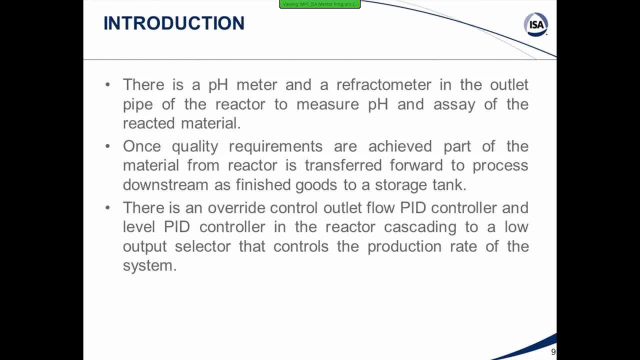 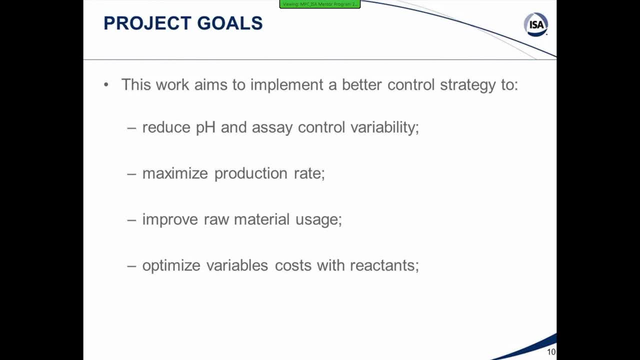 means a reduced production rate, automatically according to build up level in the system. So the main goals for this project is to reduce, implement a better control strategy, reduce pH and assay, control variability, maximize production rate, Improve raw material usage and, of course, optimize costs with reactants. 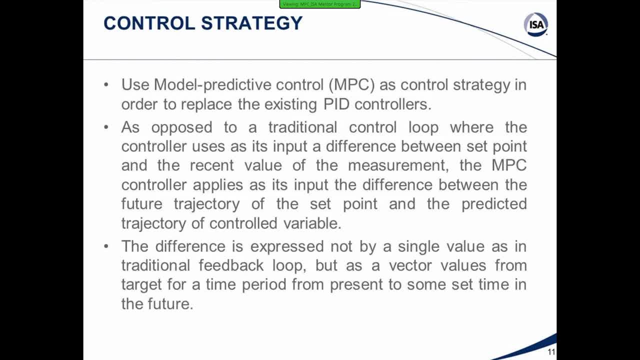 And, as I said before, the PIDs were not running properly. So, as we have a huge downtime in the process because we're running two tanks, we decided to use model predictive control, the MPC, as country strategy in order to replace the existing PID controllers strategy. 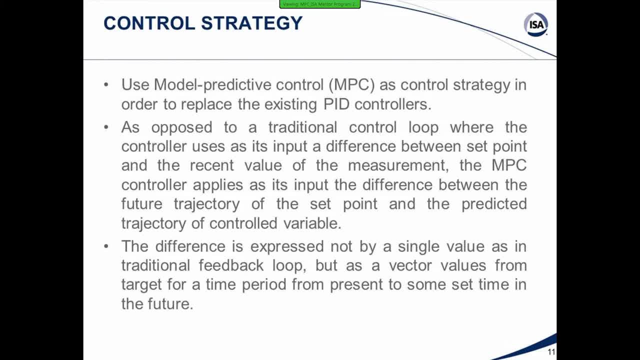 So, opposed to traditional control loop, the MPC controller applies as input the difference between the future trajectory of the set point and the predicted trajectory of a controlled variable, And the difference is expressed not by a single value- Okay Okay- Like a PID does, but as a vector of values from targeting to for a time period from present. 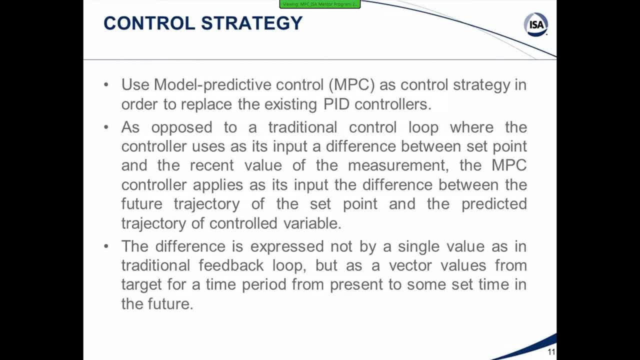 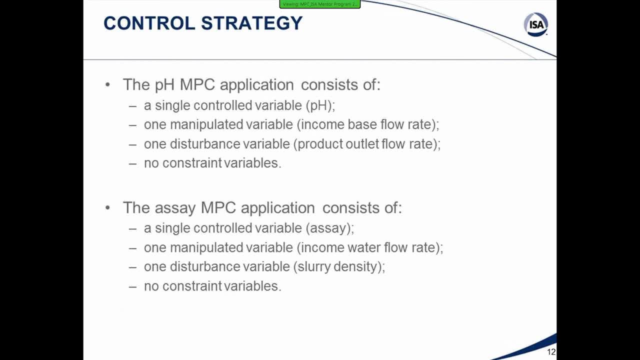 to some time in the future. So before we start building this strategy or evaluating the strategy in our cancer system, first of all we studied a little bit the process to understand what kind of variables have correlation with us. So, for example, the PIDs are the same as the control loop, but with a little bit more. 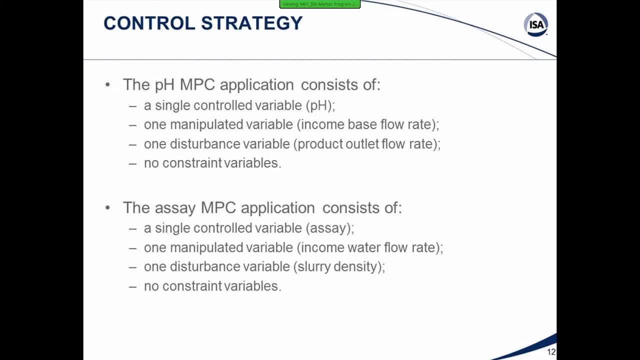 of a correlation with the controller variable. So for pH, for example, we identified that controller, of course, is pH manipulated variable, is the flow, the base flow rate and the reactor, And we find out a disturbance variable, that is the product outlet flow rate. 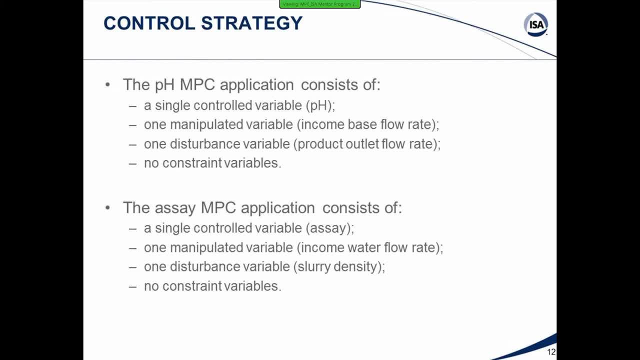 And we didn't identify any constraints- variables for this system. pH could be, but we decided to go with the product outlet flow rate And we decided to go with the pH. And we decided to not use that because when pH is off spec, we do not send it to downstream. 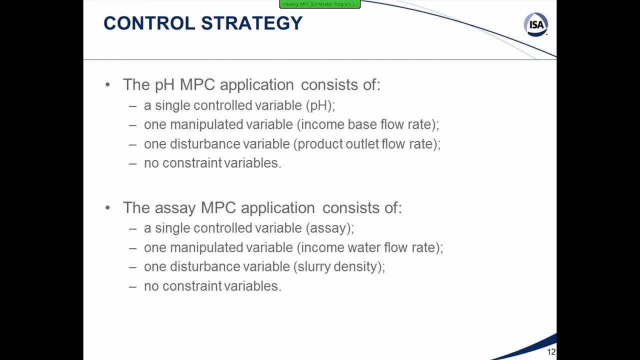 So for the assay MPC application, we are controlling assay, manipulating the income water flow rate in the slurry tank And we found out as a disturbance one the slurry density. So the density is measured in the transfer line from the slurry tank to the neutralization. 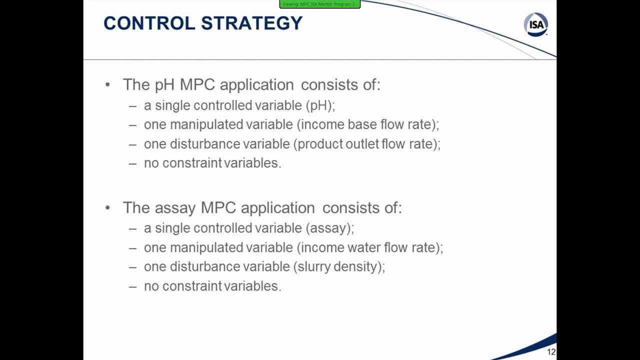 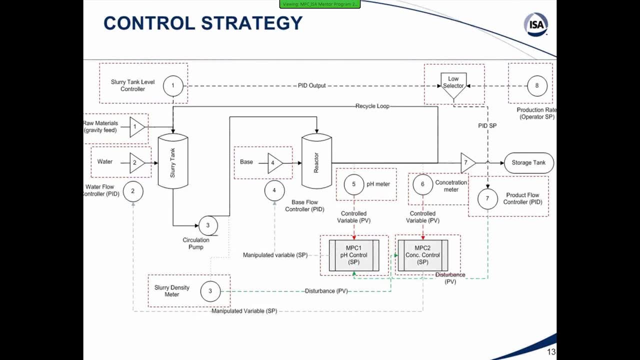 reactor, And also we didn't find any constraint variables for this strategy. So what we did first was we – this is the first step- We look at the existing control strategy. So the number one here in the chart, the slurry tank level controller. 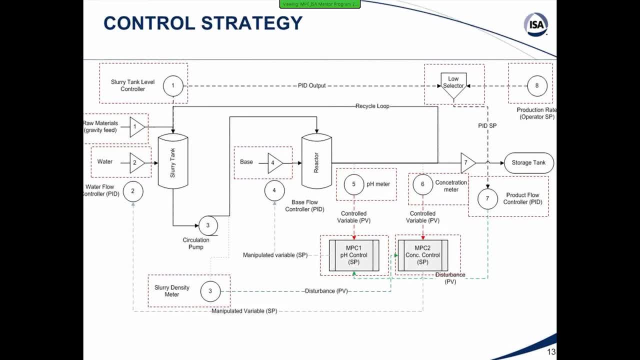 So it look at the level inside this tank, that's – it's controlled around 60 percent. The reactor is – skip 100 percent level, So it's flooded. And what it does is – the operator sets the set point required for the production rate of the plant. 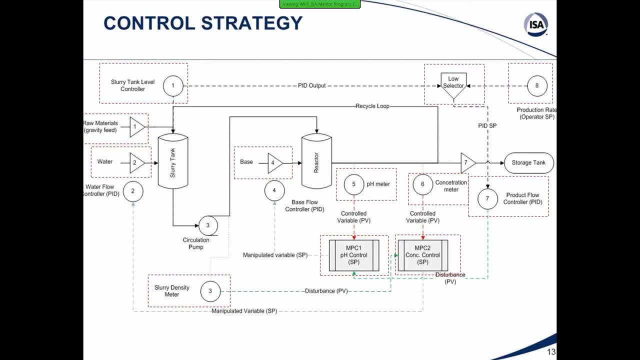 So it's number eight here. Then we have an over-height controller with a low selector here that is going to get the lower – low value from both – from the level control and the operator set point And set the set point for the product flow rate: PID controller. 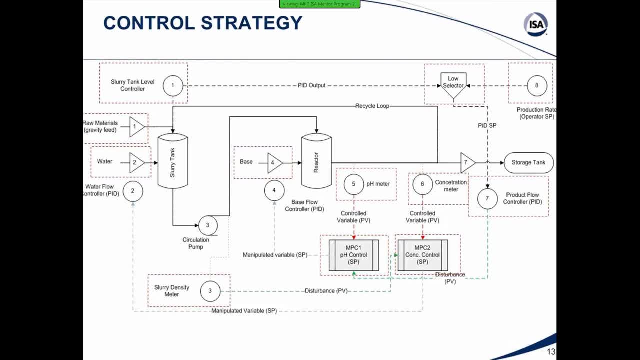 So – This is – This is to keep the operation stable and keep a certain amount – a minimal amount of product in the system to guarantee a good mixing and also a good reaction and residence time. So then, we developed the MPC-1.. The MPC-1 is the pH control. 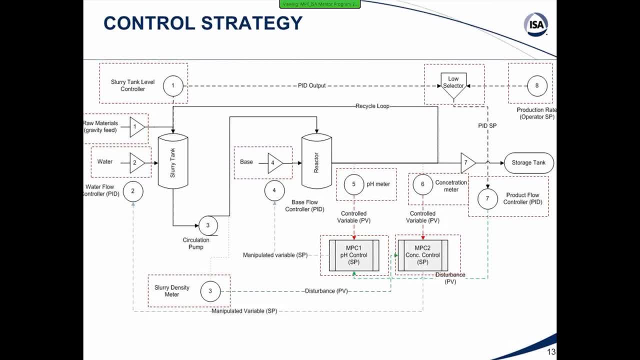 So, from the number seven, is an input The PV. The PV of the product flow rate is a – is an input for the MPC control. It's a disturbance. We have the number five, that's the pH meter. Also, it's another input. is our controller variable, in this case? 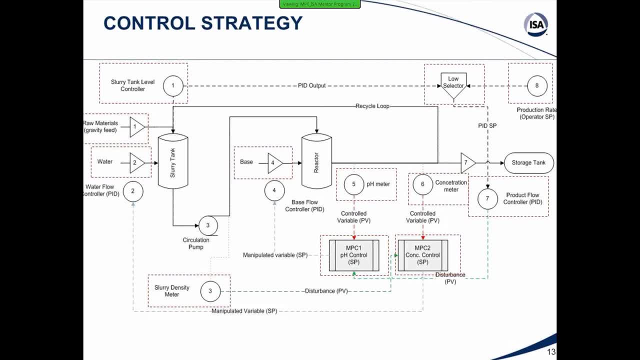 And then we have an output from the MPC to number four, to the base flow rate PID controller. So in this case, the MPC – The MPC calculates the set point for the base flow rate controller. It's a – it's a PID controller, a regular PID controller. 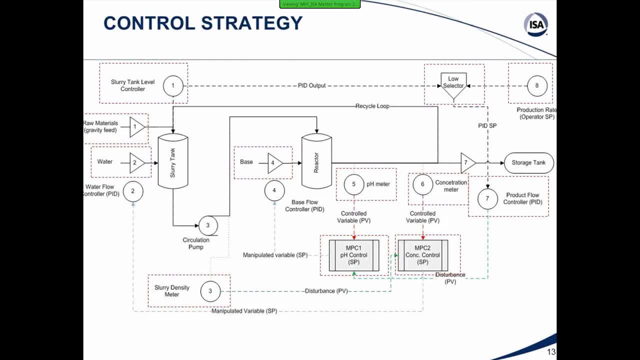 So for the MPC-2, it's a very similar strategy. We get the concentration or the assay meter. the refractometer is the number six. It's an input to the model. Also, we get the glory density meter: It's a number six. 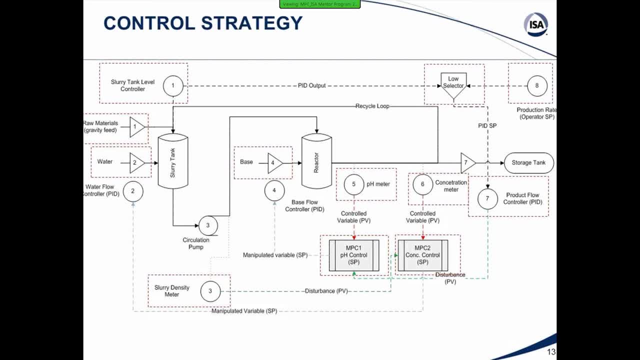 Then we get the PID 2.. Number four: It's an input, It's a DEC as a key player in the system because it compensate level, pH and production rate, so as we increase production rate or reduce level in this tank, so we keep the 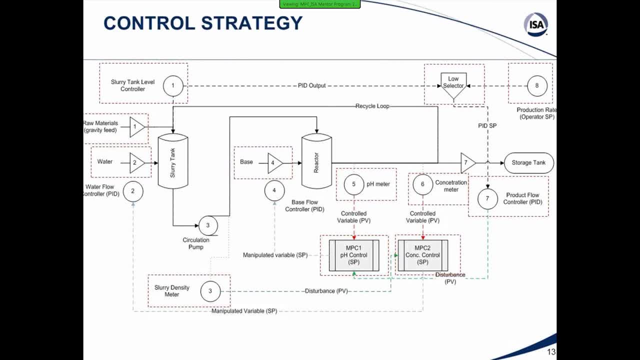 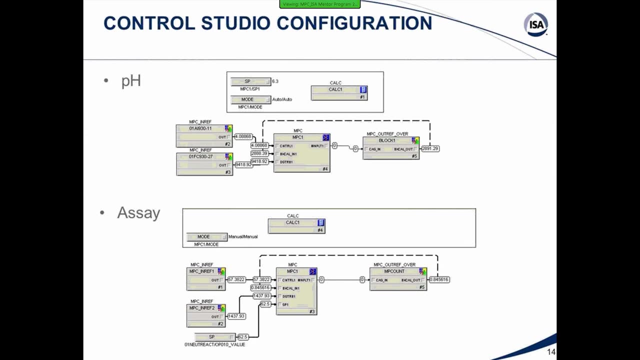 enough valve open for a longer cycle so we can feed more solid or in this this Larry tank. okay, all right. so to develop the PID strategy or the MPC strategy- sorry, we use of the counter studio configuration. this is a to available in our country system. so it's principle the we link the MPC block with. 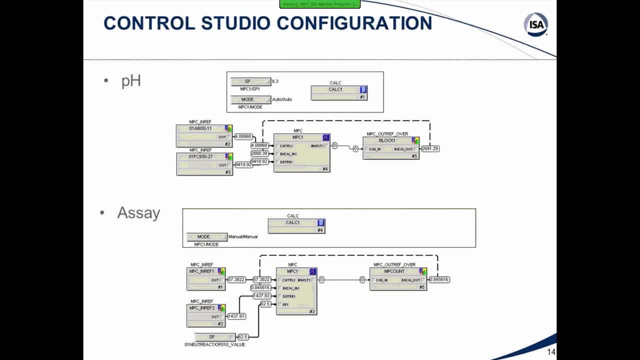 the inputs and the outputs and also with um, um, the set point required. Normally the set point is a variable that the operator can change And also for the assay we do exactly the same, of course with different inputs and different outputs, but the strategy is very similar. So when we do it in the counter system, 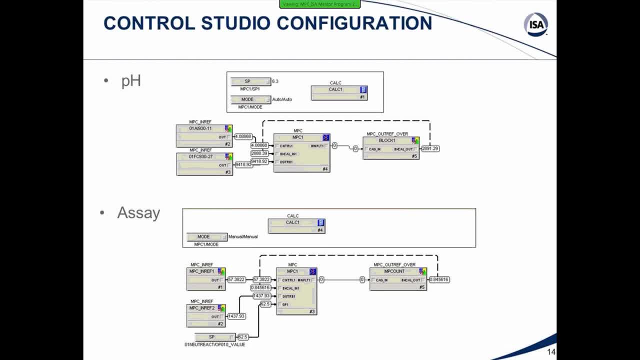 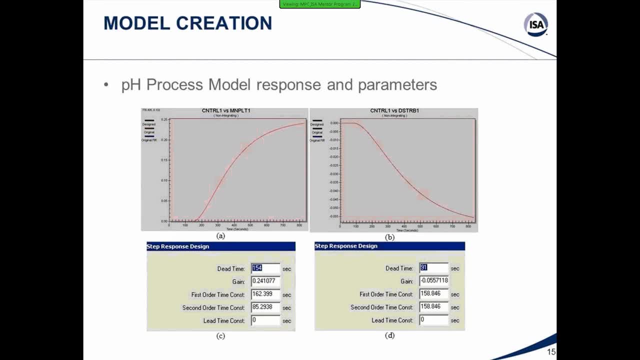 and we download it to the controller, then you are ready to start building your model. So the next step is build the model. So to do that, we can do it in either way, automatic or manual ways. In our case the tool. what it does is make some step changes in the manipulated 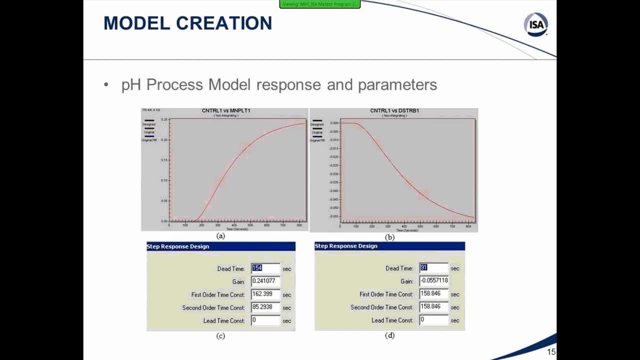 variable and we record the historical data and then we get the peer-reviewed data. So this is the period that we use it, the test period to generate the model. Other ways to give manually step change in the manipulated variable up and down. So you are going to. 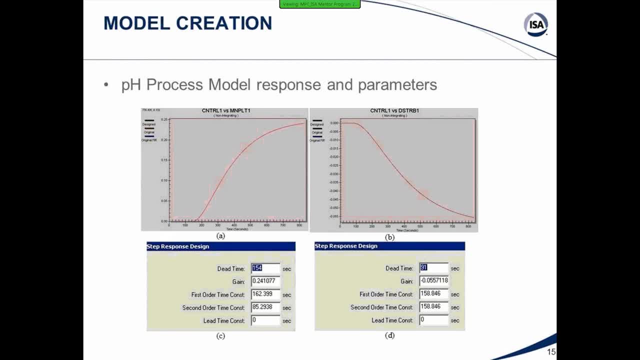 run the test for a certain period of time, and then we collect the historical data and also generate the model. So you can do either and it works, Okay. So what our tool does is collect the information and generate the process response or the model. 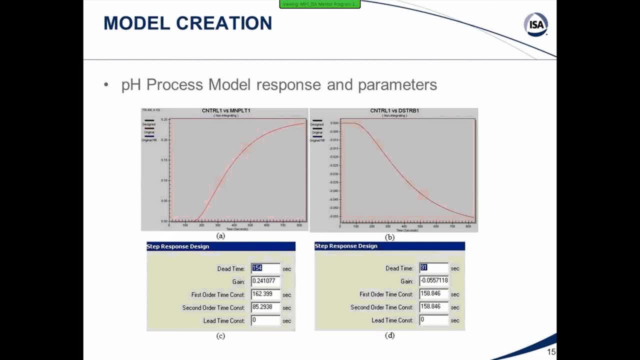 response. So in this case you can see the controller versus manipulated For the pH, the first thing we need to do is to make sure that the gain is in the right direction, if it's positive or negative. In our case, it makes a lot of sense if you increase the base. 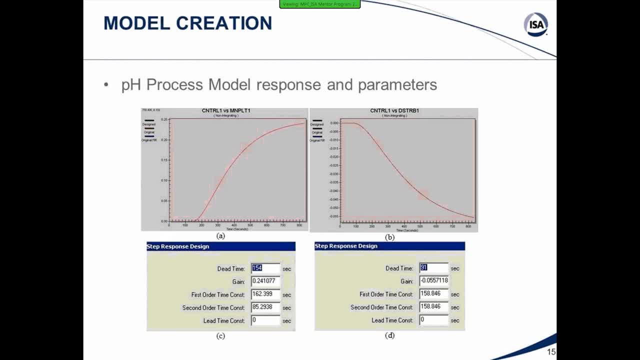 flow rate, Of course the pH is going to go up. On the other hand, if you increase production rate, the pH goes down because we let the solids- more solids- to come into the slurry tank and it drops the pH significantly. So this is one first. 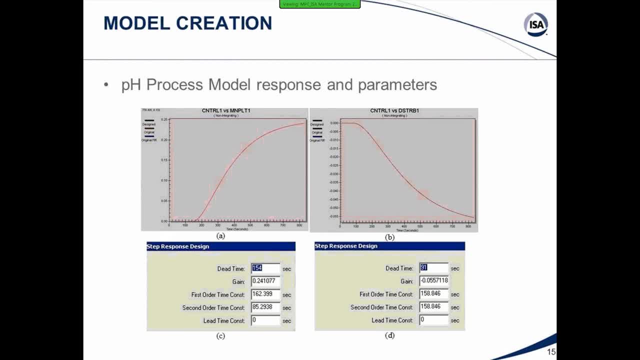 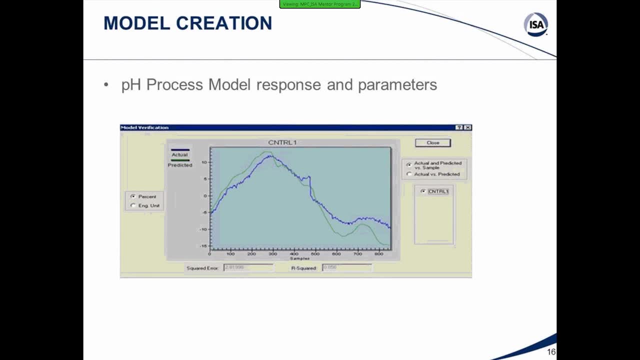 evaluation that you should do Also. the next step is to compare the echo measurement with the predicted. I mean, when you get and generate the model, what it does is compare what the model is predicting against the actual data And of course you're going to have some error, but the minimum, the error. 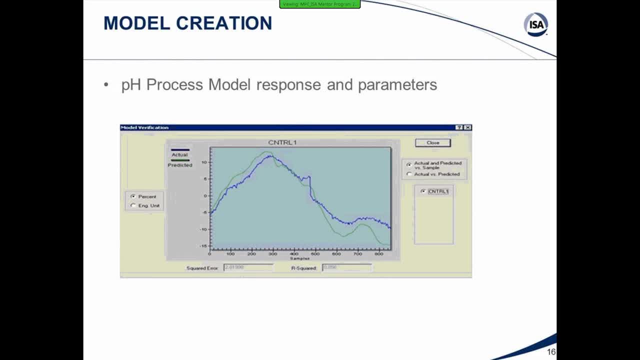 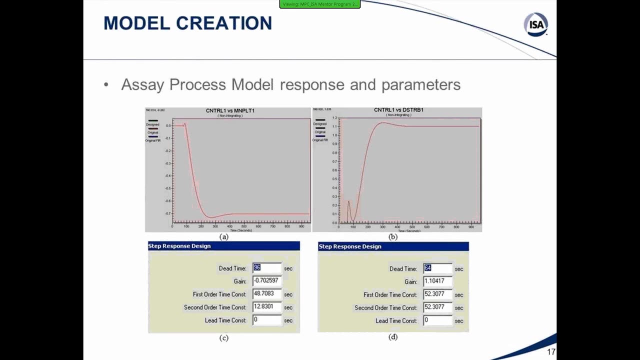 is, the better the control is. So in our case we get a very, very good model with low error for pH. Okay, For assay, we did exactly the same. In this case. we ran the tests separately. First we ran the pH tests on the plant. 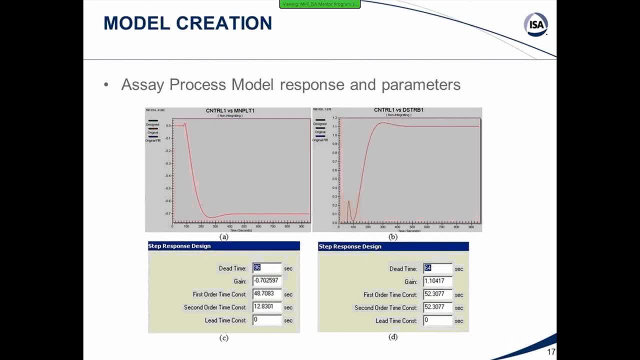 In a different time we ran the assay tests, So in this case what you can see also is the response of the variables. So talking about controlled versus manipulated makes a lot of sense. If you, If you manipulate the feed rate or increase the water feed flow rate, the assay goes down. 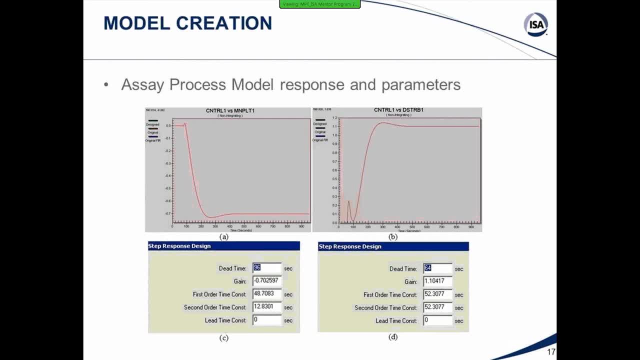 So it's a negative gain. When we talk about disturbance, that's the, in this case the slurry density. As the density goes up, the assay goes up because you have more solids in the system. So when we finish that, the next step is to compare the assay results. 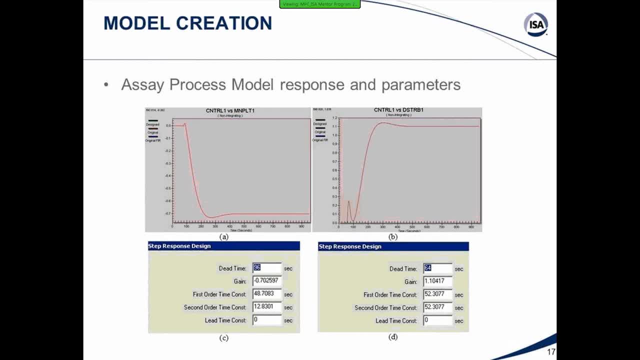 So when we finish that, the next step is to download the model to the controller, to the MPC controller, and start testing, make some tests on the plant to check the performance of the model and if you have to need to adjust any variables or need to retest again. 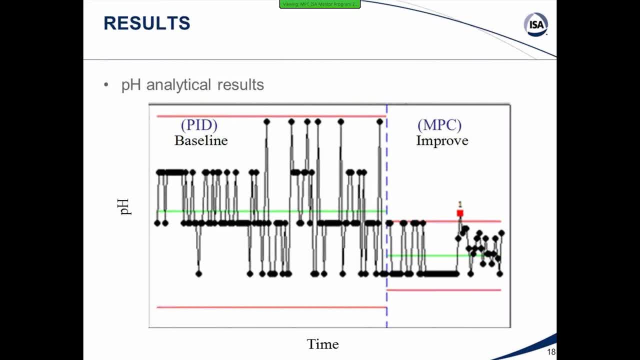 So in our case, our result: we got some samples from the plant Okay- And we analyzed them offline in the laboratory. So we took every three hours samples for pH analysis And if you look at the baseline when we were using PID controller, we have a bigger variability here. 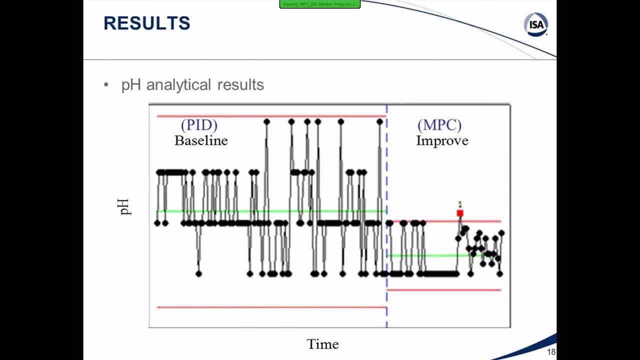 a larger variability and when we moved to MPC we reduced the variability and also we had a chance to reduce our set point, So we minimized, We reduced our set point closer to the specification target, So this provides a lower consumption of reactants or base to neutralize the product. 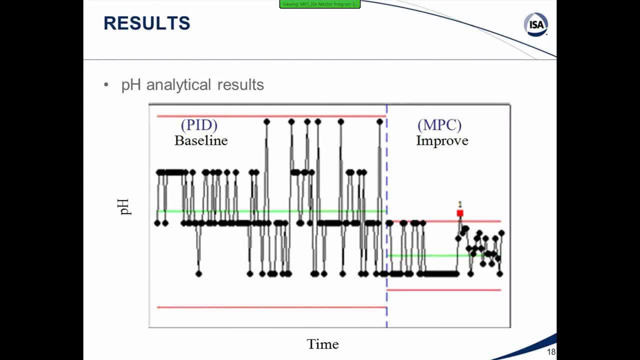 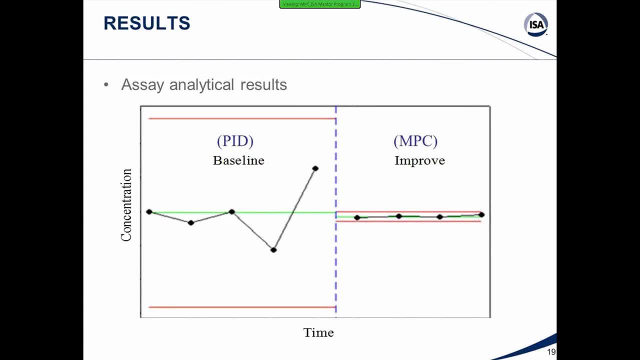 and, of course, reduce cost. with raw materials consumption For assay, we observed the same results. So the PID had a large variability- It's very large actually- And we We started the MPC operation. We observed a very, very low variability. 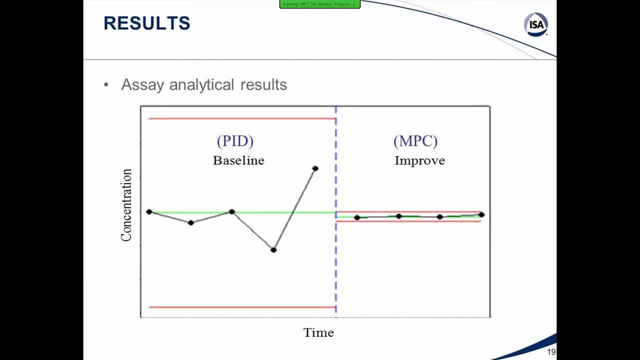 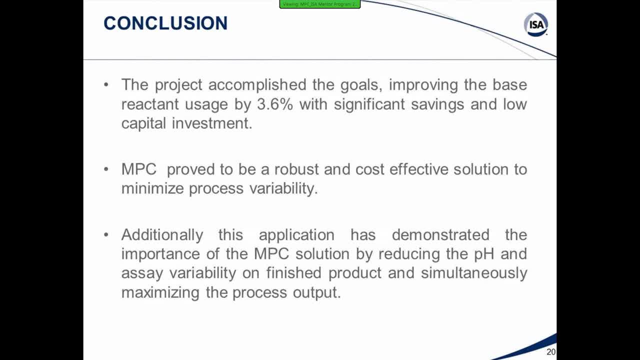 So, concluding this, We could save around 3.6% of total base reactant consumption, so it brought us significant savings, and with very low investment. Actually, we only spent some A few hours from our engineers- process engineer and process control engineers. 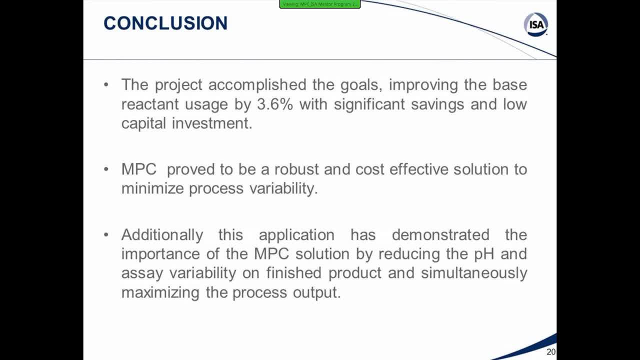 Okay. Also, the MPC proved to be robust enough and cost-effective enough to minimize the process variability and also maximizing the process output. Once we narrow our range, our operating range, we could avoid, for example, we have many down-times in the plant because of high or low pH or high or low assay. 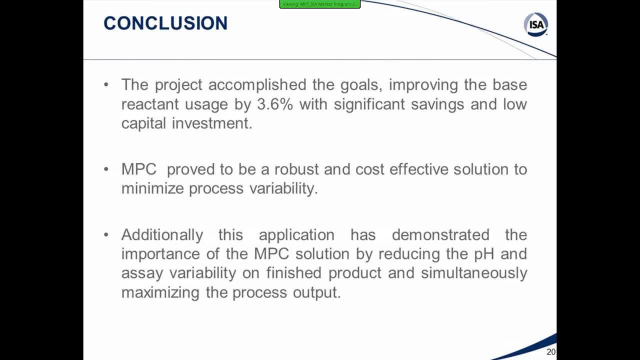 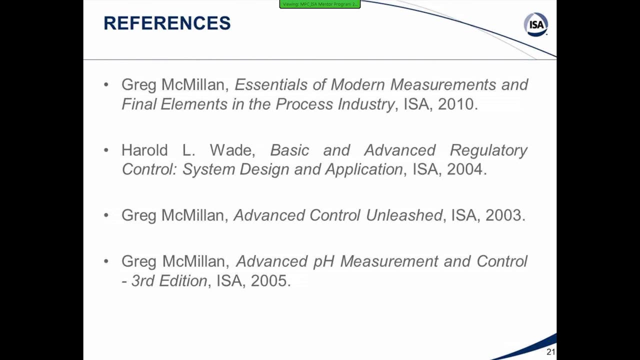 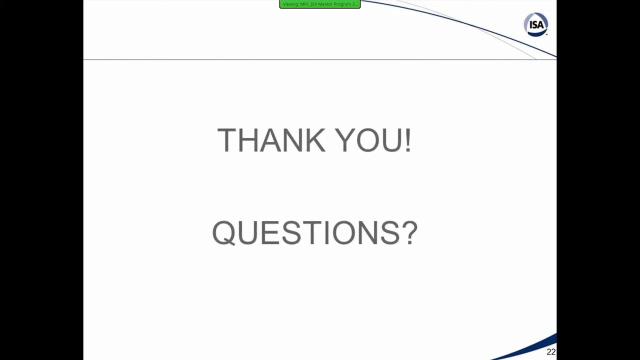 In minimizing variability. we reduce that and keep the plant more stable and pushing up the production rate. So the reference that we use in some books: it's good to read them because you get more information about the application and also the concept. Thank you for joining the call and if you have any questions or comments, feel free. 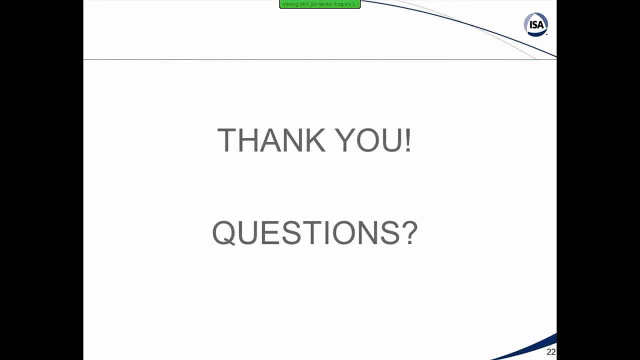 to do that. Yes, good afternoon. This is Bart Probst. I was just wondering how long did it take to deploy the application from concept to commissioning? All right, We spent around three weeks. The first week was the definition, or the design, where we evaluate all the process variables. 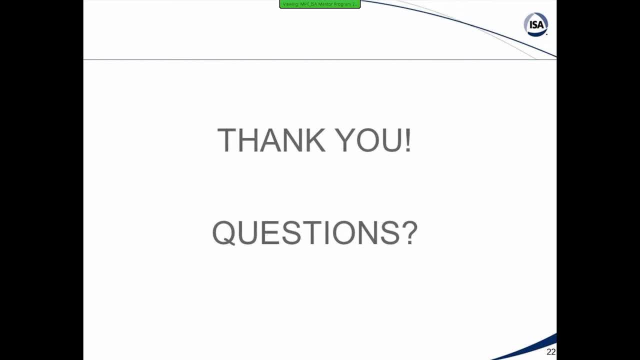 We look at which ones have correlation with the other ones, especially with the controller variable. Then after that we selected the variables and we start thinking on the control strategy itself. So we spent the first week defining. So we spent around three weeks. 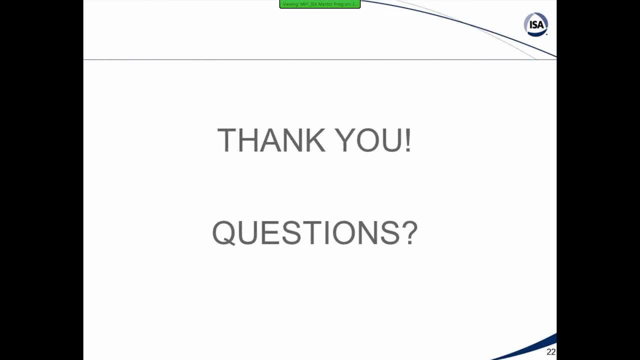 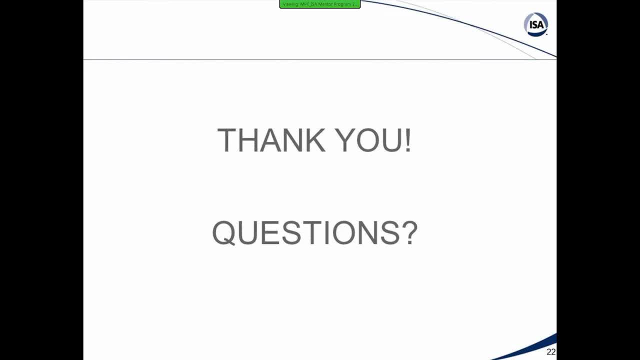 planned tests And the third week we put in operation and we monitored the performance for adjustments or maybe to retest in case there is a problem. In that case it fails or doesn't work. So actually we spent three weeks. 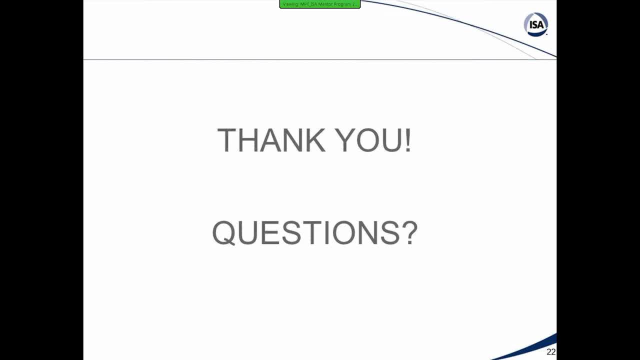 And I didn't tell that before, but we have three different products and we had to build one model for each product. So we have three different models for pH and three different models for assay control. All right, Thank you very much. 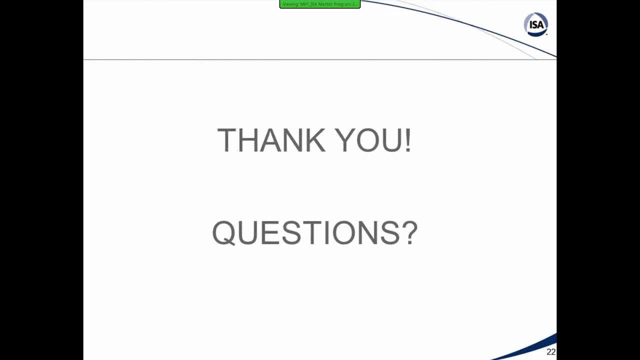 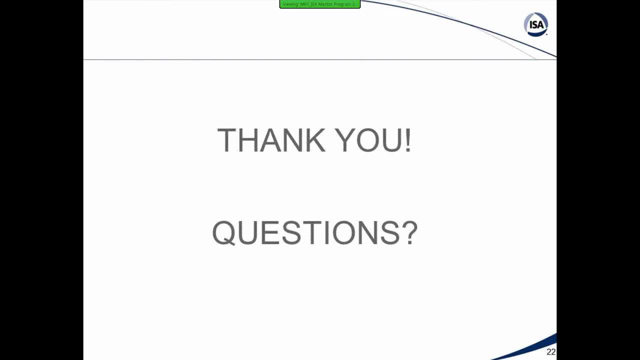 automate to make contributions to the team, because normally the operators know more about interactions between variables and and, but of course we use some statistics to determine that, but also collect their operators feedback to avoid wasting time, right, right, and then can you give me a feeling for your? 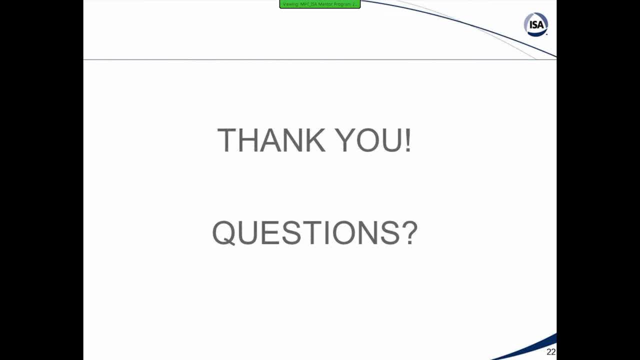 experience level with the APC applications in deploying those. yeah, this model that I presented here, we, once we get the model done, I put in operation and the first first impression was very good and since then we implement that three years ago and since then we have been working, operating the blank and we haven't been 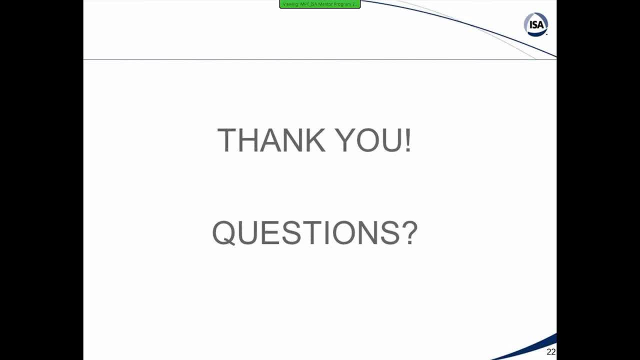 touched the model yet, so it's performing as the first day of operation. so my impression of MPC operation is that it's very, very robust too, and and and if you don't have problems in the field with some instrumentation or equipment, you don't need to touch the model, the model. 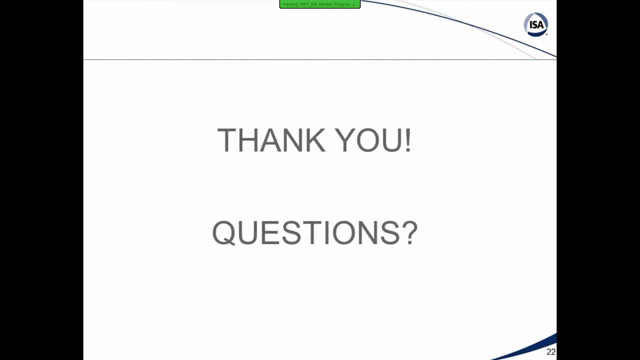 is very: keep stable for for long period of time. okay, thank you. yeah, if I'll be a quick question here, this is Devin Marshman. did you do anything to linearize control around pH? like it's, it's highly nonlinear, so I'm just wondering if you did anything there. no, no, no, we just we just look for to do. 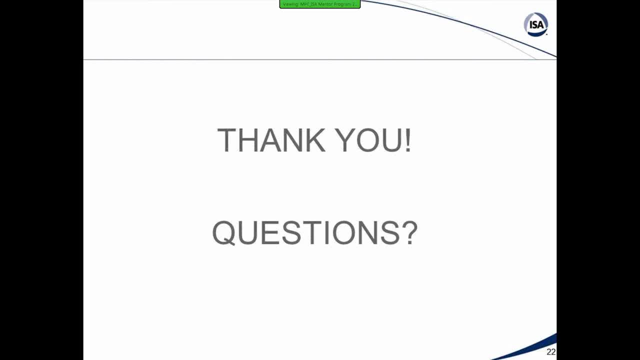 the test is. what we decided to do is to cover the full range of pH that is required for, for to meet our product specification. so from the lower specification limit up to the higher high specification limit and for for our products, the range is very narrow. so and it's in, and it's below seven, so it's in a point that is more. 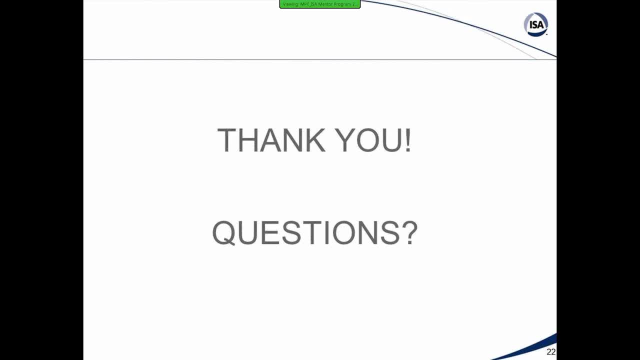 linear than when you have switched from acid to base pH. so in this case it's a. it's a kind of more linear range, but we try to covering in the test the full range just to get a perception or if you have difference in the game, you could. 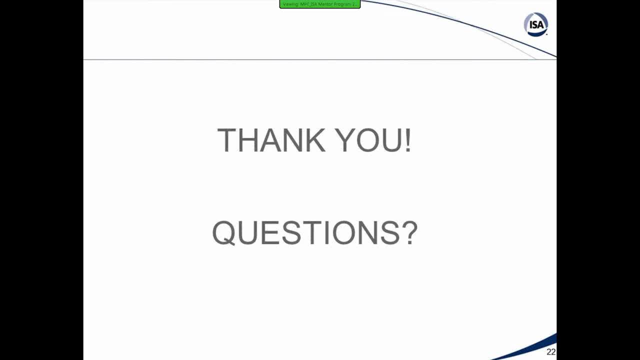 observe that during the test and and on the behavior of the variables themselves. okay, thanks. So in case for the manipulator, and what we do is we did a kind of five percent step up and ten percent step down, and and we did and repeat that like three, two or three times. 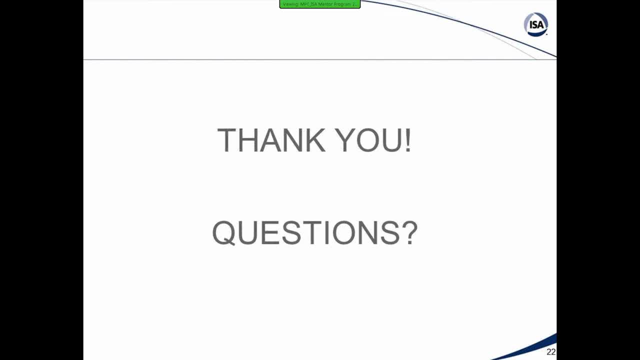 so we record those data, the historical data, and then we generate the model based on the period of the test. Okay, Okay, Okay, Yeah, Very good. I would add that by doing tight control, you are operating on a smaller part of the titration. 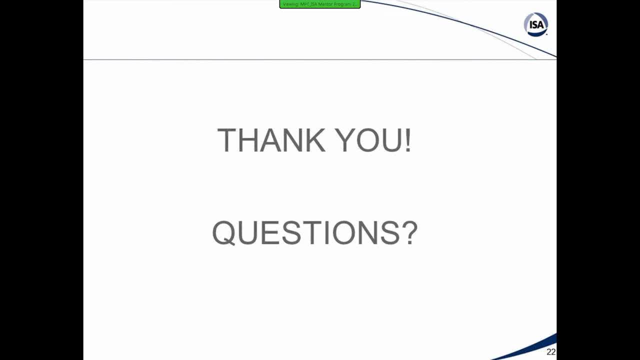 curve, which Flavio alluded to, and so you don't have as much of the non-linearity. so it's sort of like the better control you can do, that less non-linearity. it's going to see, and it's sort of self-effective. 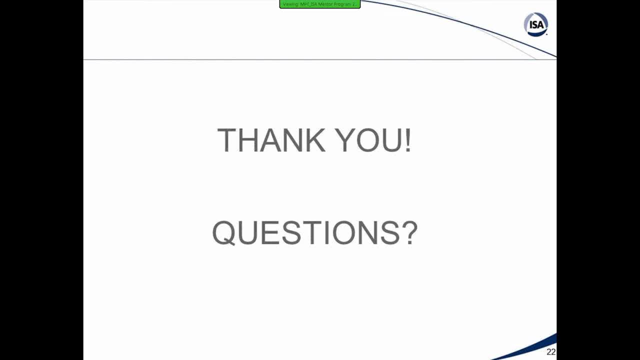 Yeah, I guess I'll throw a question out there for everyone else on the call is: do you all see any other any applications for in your own places for small NPC controllers? Yeah, Actually, we implemented recently an NPC control for steam to control steam flow rate in a. 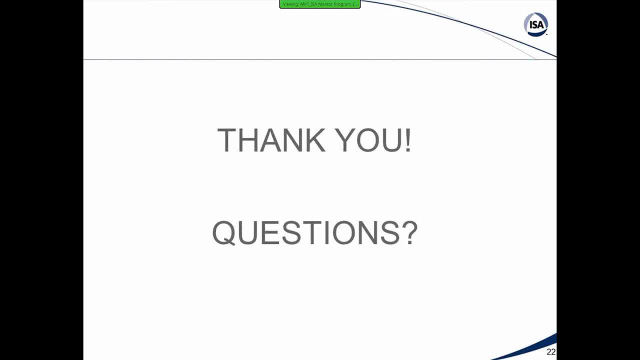 thermal compressor for an evaporator, So, and we in this case we had an upstream batch process and you had to convert the variables into a kind of continuous flow rate. So it's kind of continuous variable in order to determine the hydraulic load that's coming. 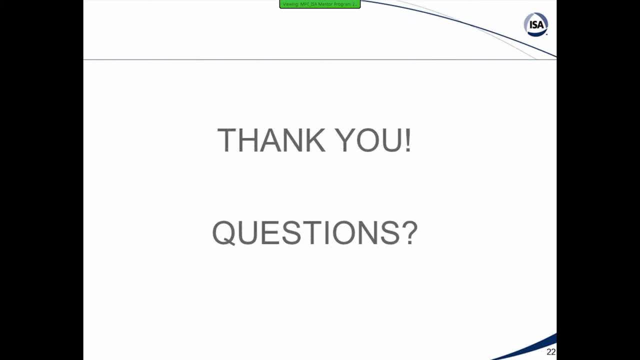 from upstream process and also the NPC drives how much steam we need to evaporate and keep the evaporator level more set. So this is another application. I don't have the slides here, but I can present it to you, Okay, So it was really interesting because we saved a lot of money with natural gas and because 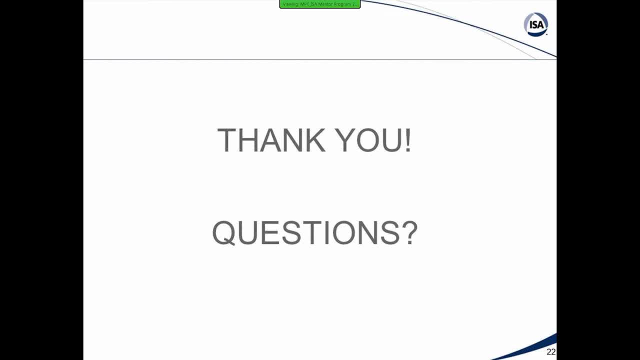 we burn natural gas in the boilers to produce steam and we reduce 10% steam consumption just manipulating the steam flow using an NPC. So it's another application that we have been implemented in the client And it's running very well up to now. 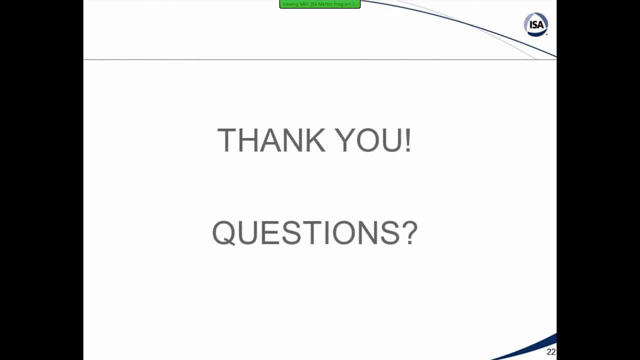 Great. Thank you very much. I think one point to reiterate is that the MPC, the small MPC, was built into the DCS, so it was just a matter of doing the configuration and dragging and dropping those blocks in to Control Studio. 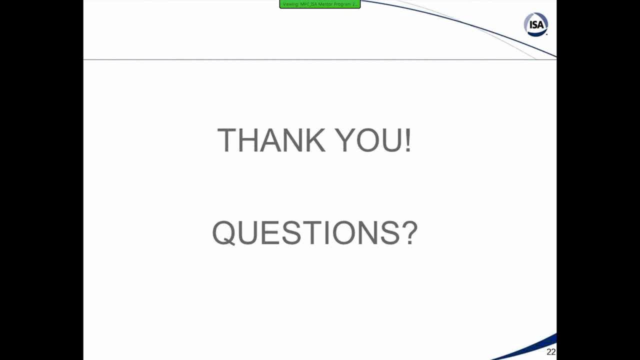 So, Flavio, did you have to do much input or output conditioning for your MPC blocks on your inputs? Yes, for example, we have some constraint range for the variables, Because in some case, when we have, for example, we drive, for example, the manipulated variable, 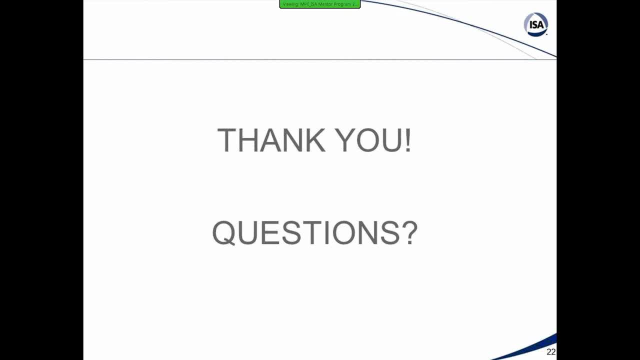 I know that we have a maximum flow rate that the process can get for each type of base that we use. So what I do is I put a constraint that limits the maximum flow rate and the minimum flow rate In order to avoid Okay. 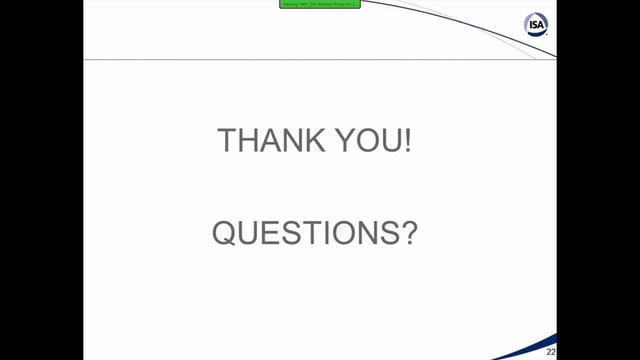 To avoid some fluctuations and strings in the control. So this helps a lot because you keep the control in a certain range and that guarantees that you're going to be more stable. the control is going to be more stable And for input, what I do is a kind of treatment in the data like don't get negative values. 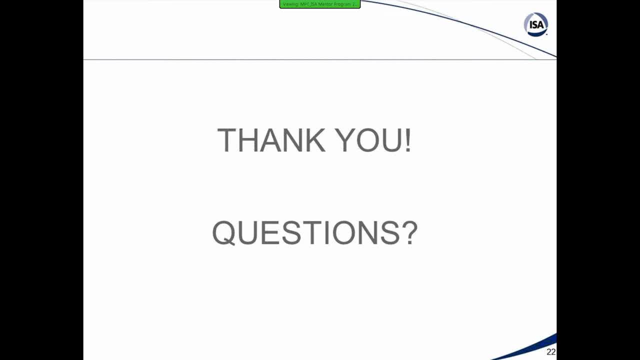 or something like that. That also helps to avoid any issues. I don't know if I'm not sure if I've answered your question, but that's what. Yeah, Flavio, this is Maudela. Yeah, just had a quick question. If I remember right- I think you mentioned you had three different modules. Yeah, Okay, Okay. So you had three different modules that was built to run different products on the system? Yeah, Three on each, on the PH and the SA. So did you give some kind of a control for the operator? so when they changed the type, 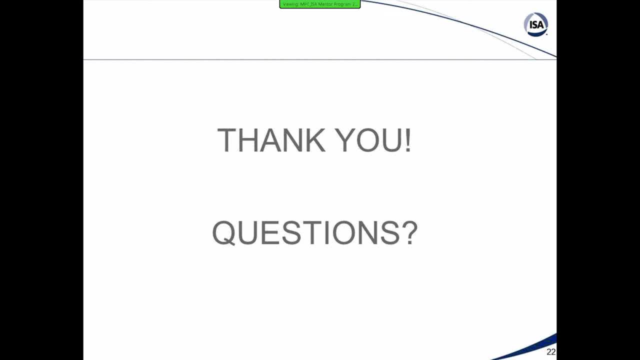 of product that it runs. did the MPC automatically change the model to suit for that time? Yes, Yes, correct. I have a product selector. So, before we start the operation, what is The operator needs to do is to select the right product he's gonna produce, and then 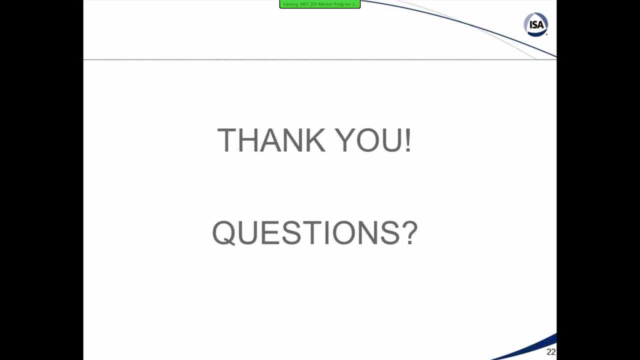 all the parameters, not only the MPC, but all parameters, set points, et cetera- is loaded to the unit and we start it run the process automatically. So we have automatically a switch that selects the right modules in Delta V. So we have a 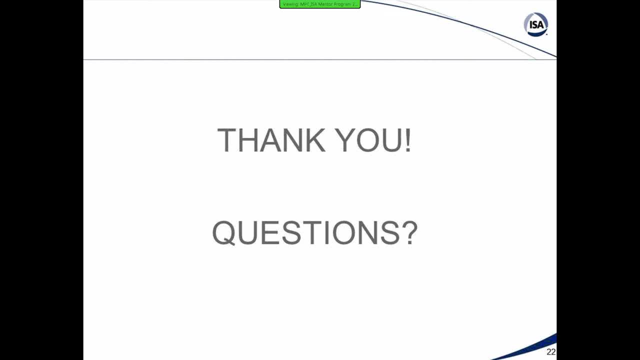 switch that selects the right modules in Delta V. Okay, Okay, Okay, Okay, Okay, Okay. And that's the whole point We have to start to make: To start the control with no problems. So if the operator does not select the right product, the system knows, because we have. 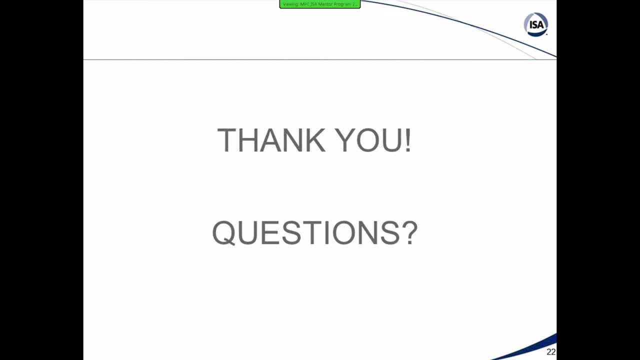 some valves, that we monitor the position of the valves with the right base. So if the product does not match the base that we are supposed to consume with the, it stops and the operator needs to make the chain select the right product. so we have some, some interlocks but some some process actions that avoid operator to 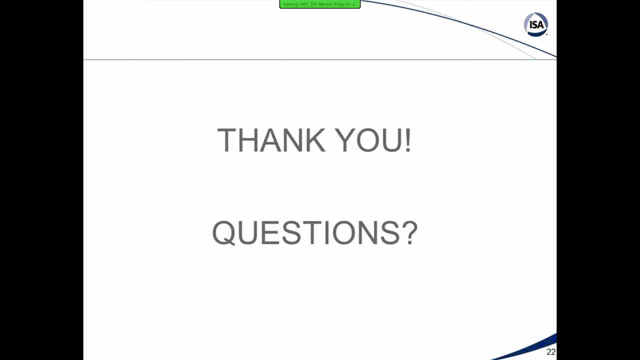 make a mistake and properly selected the right product and also the system is going to set and and drive the the correct model to the to run the controls. so in reality, like on the, if you look at it on the control studio would you actually have like three separate. 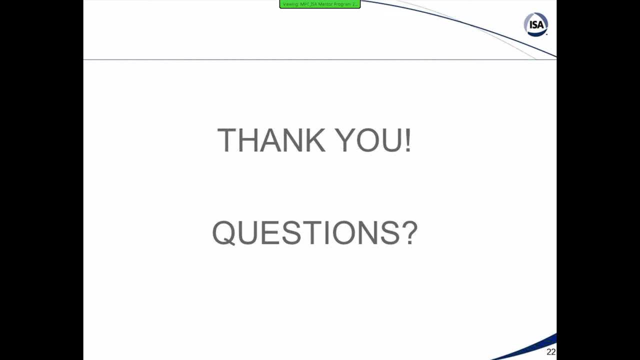 MPC blocks for the three separate models. so yeah, oh yeah, that's what I was trying to see: how it automatically loads up the models depending on the product. so thank you, yeah, we have three different modules and we select the one that we need to start a control and that's it. so 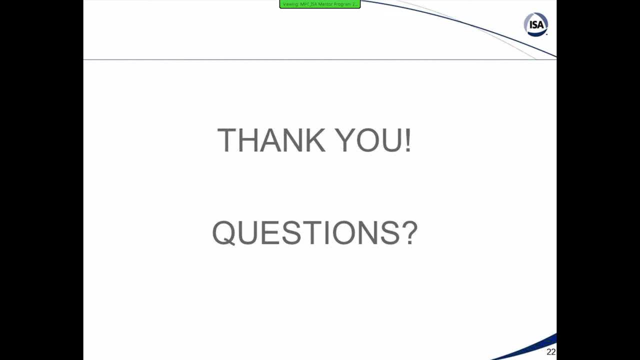 in this case that we're talking about pH and SA. we have six different models, you know: three for pH and three for SA control. okay, thank you. yeah, well, thank you. I guess we are done there. we hope to have a YouTube recording middle of next week. we.